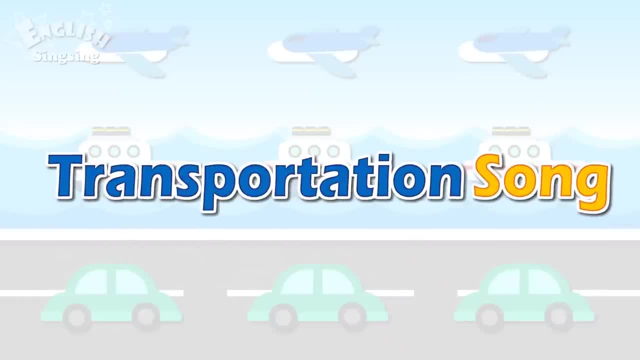 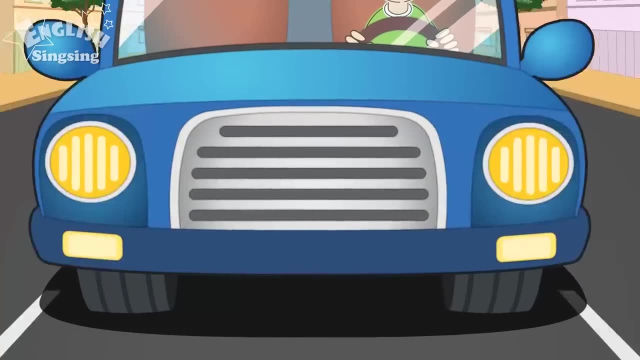 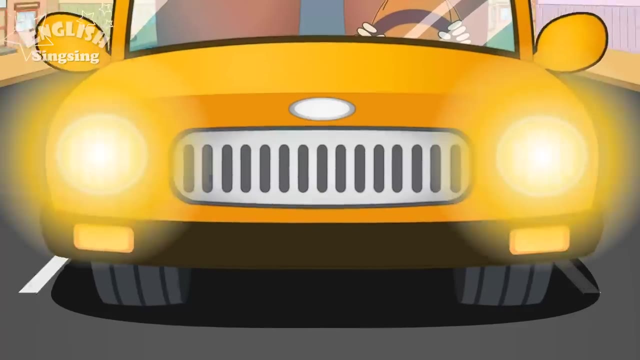 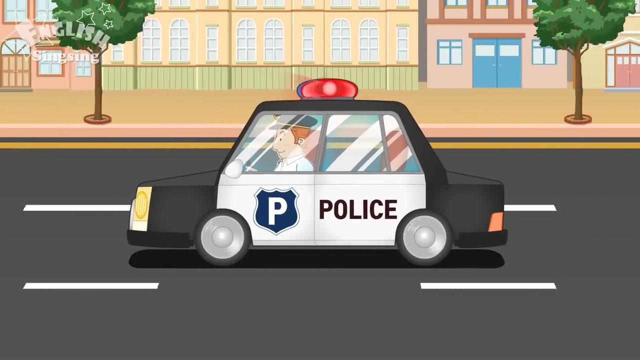 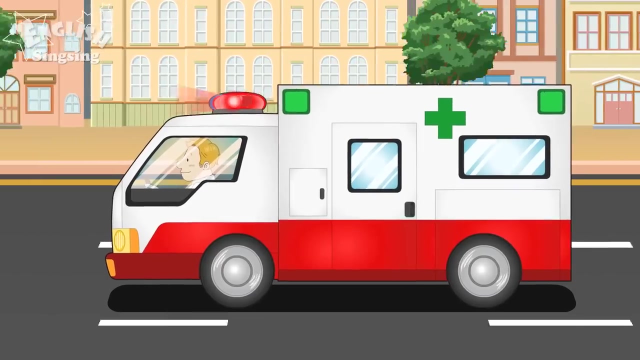 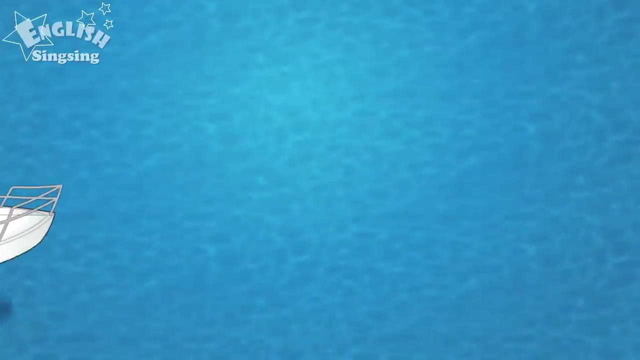 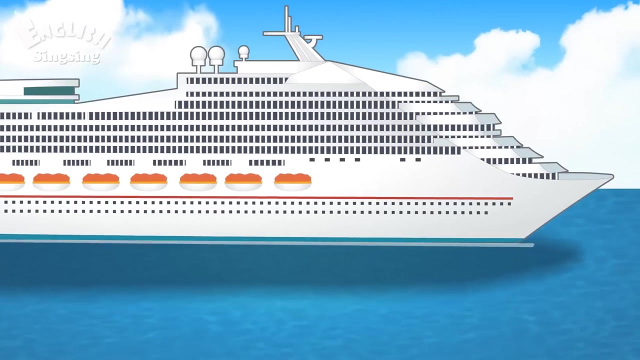 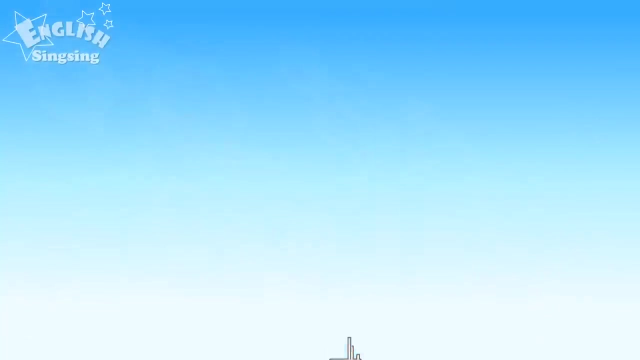 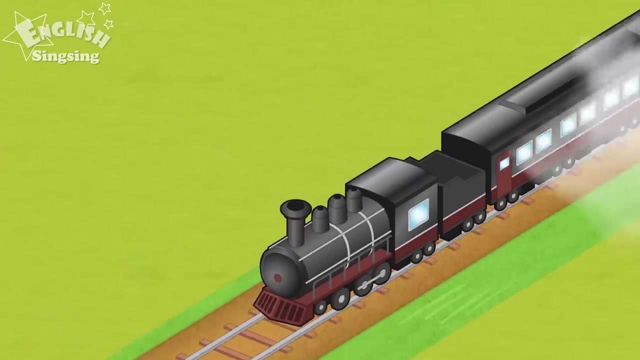 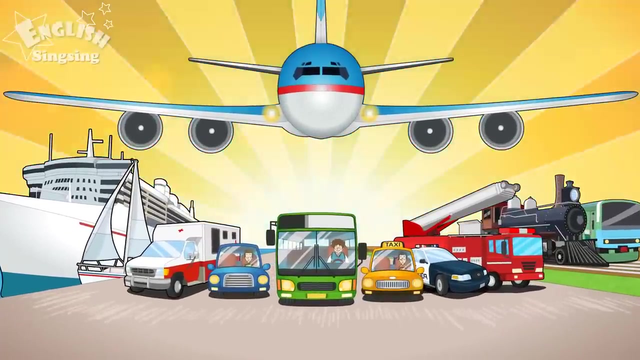 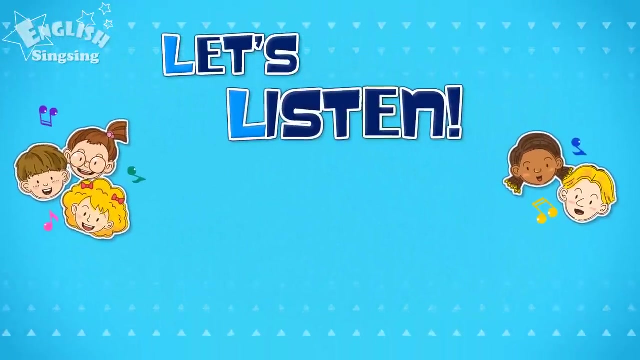 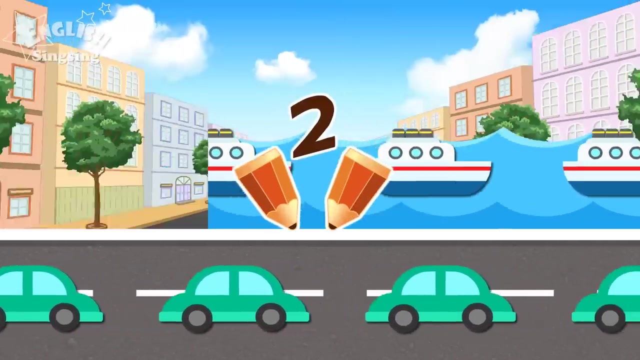 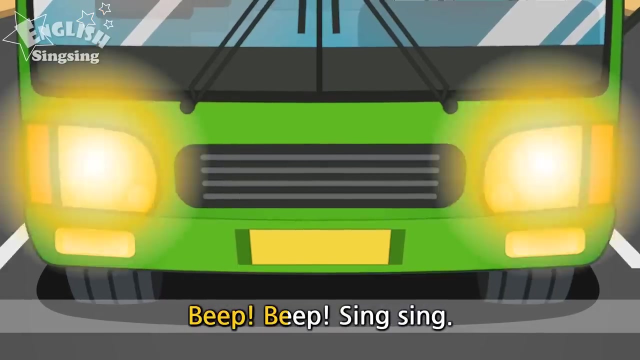 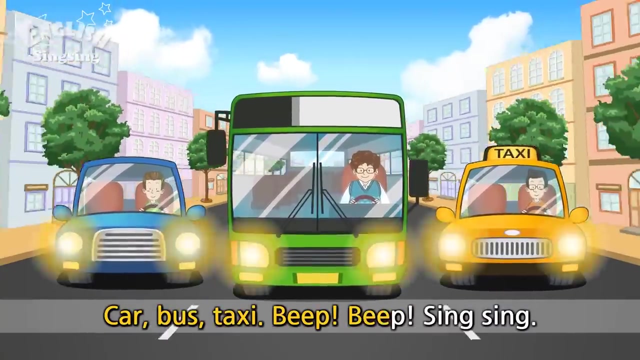 Transportation Song Ambulance Wheel Boat, Yacht Ship Boat, Ship Boat, Subway Train, Train, Train, Train. Airplane. English Sing Sing: Yeah Car, Car, Car, Beep Beep Sing Sing Bus, Bus, Bus. Beep Beep Sing Sing Taxi. Beep Beep Sing Sing Car, Bus, Taxi. 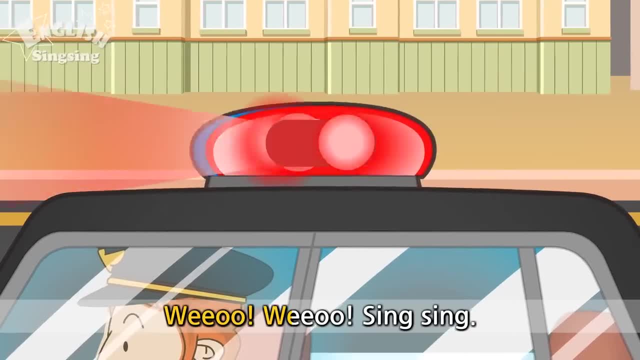 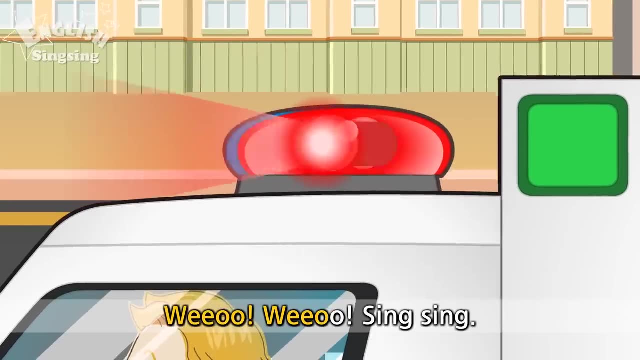 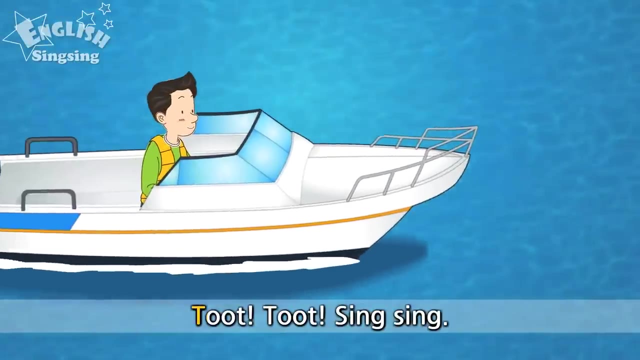 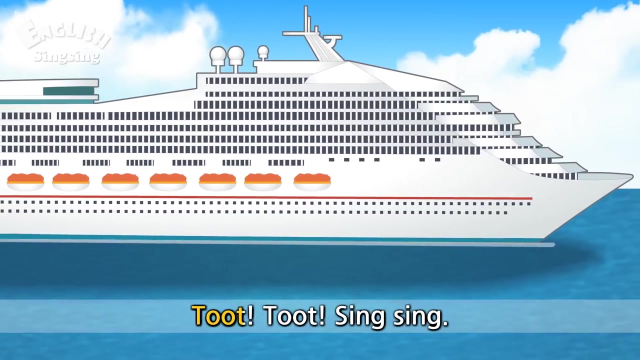 Beep, Beep Sing Sing Police, Car Police, Car Wheel Wheel Sing Sing Fire Engine, Fire Engine, Ambulance, Ambulance, Wheel Wheel Spin Sing Boat, Boat, Boat, Tute, Tute Yacht Yacht, Yacht Toot toot sing sing Boat, yacht ship. 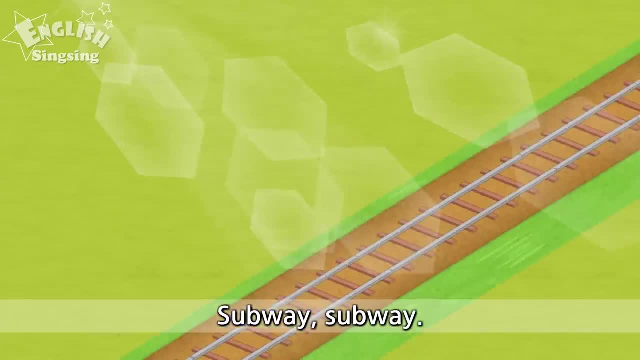 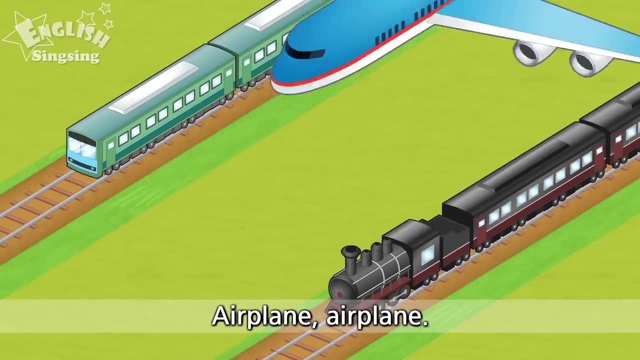 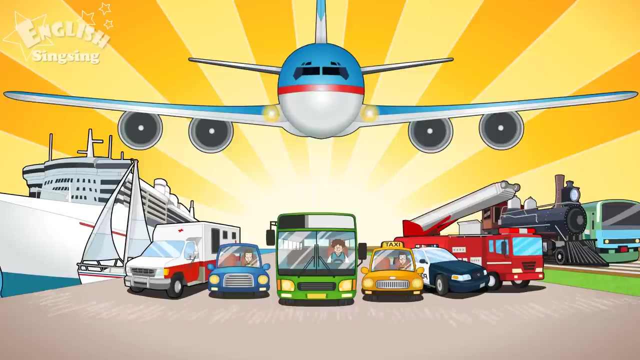 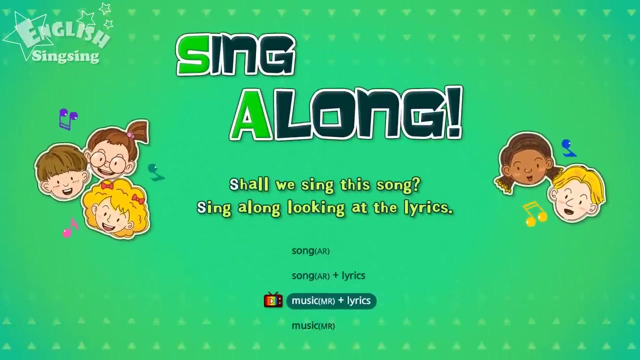 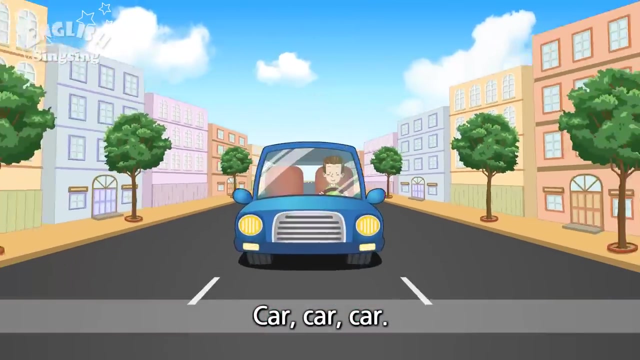 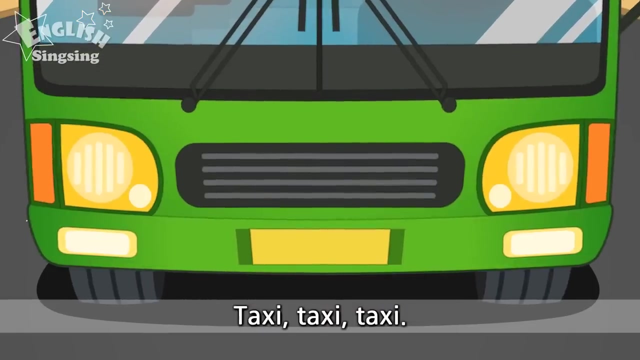 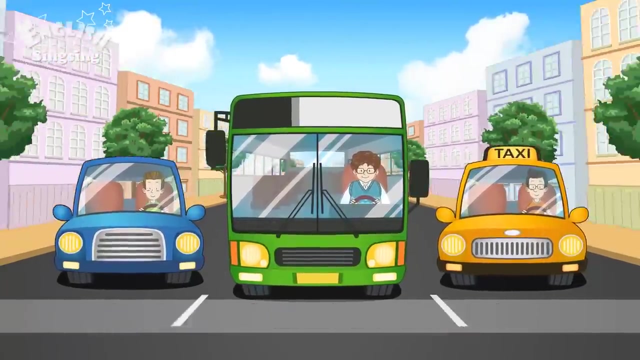 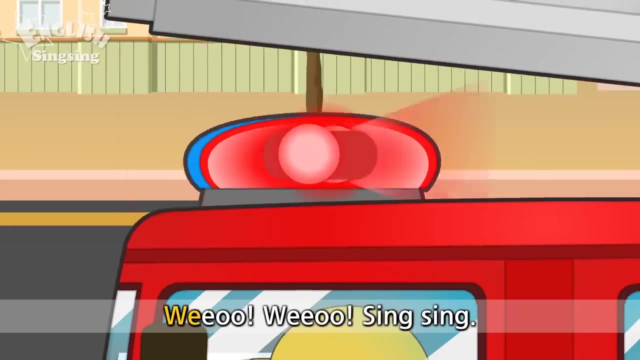 Toot toot sing sing Subway, subway. Choo choo sing sing Train train. Choo choo sing sing Airplane, airplane, English. sing sing, English sing sing. Yeah, Toot toot sing. sing.